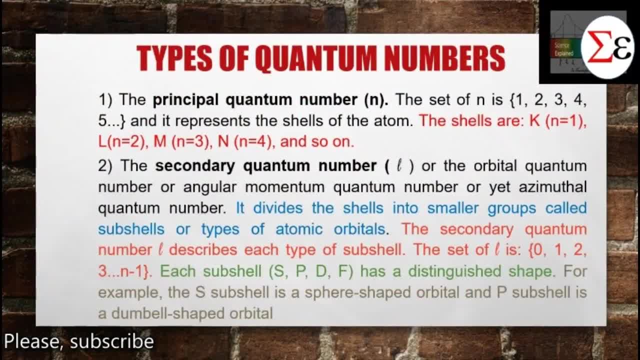 The principal quantum number n, whose set of discrete numbers is one, two, three, four, eight, nine, ten and eleven. Only ten are discrete. The person of the set of discrete numbers should be e,1 and the person of the set of discrete numbers. 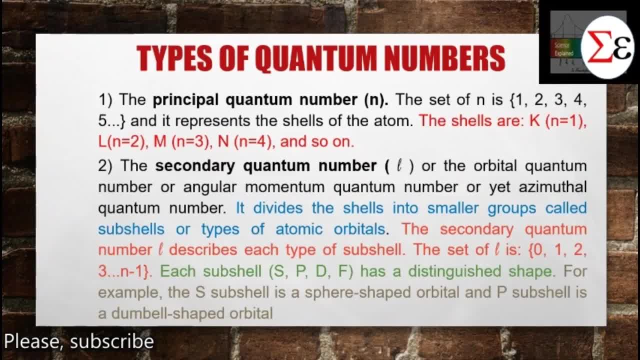 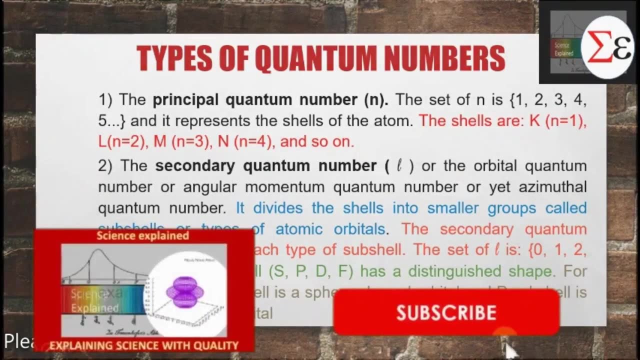 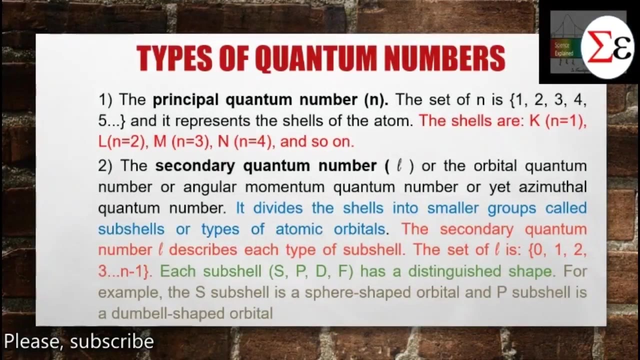 should be q and okay, do not forget the FREE link between the hashtags to learn and activate the system's機kal engines. four, etc. and represents the shells of the atoms. like uh, it was also known in the bohr's theory, the old quantum theory. the shells are k, n is one, l, n is two, m, n is three, n, n is four, and so on. the 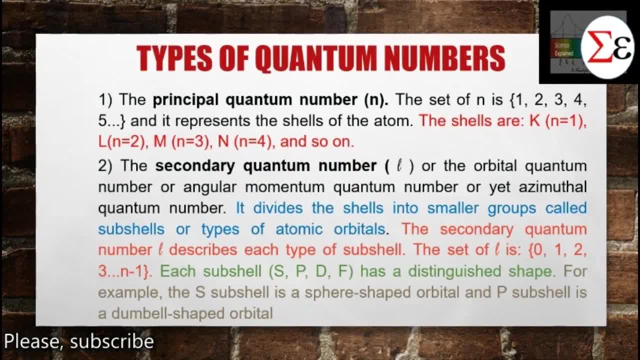 secondary quantum number l, or the orbital quantum number or the angular quantum number or yet azimuthal quantum number, divides the shells into smaller groups called subshells or the types of atomic orbitals. the secondary quantum number l describes each type of subshell. the set of l is a set of discrete numbers beginning. 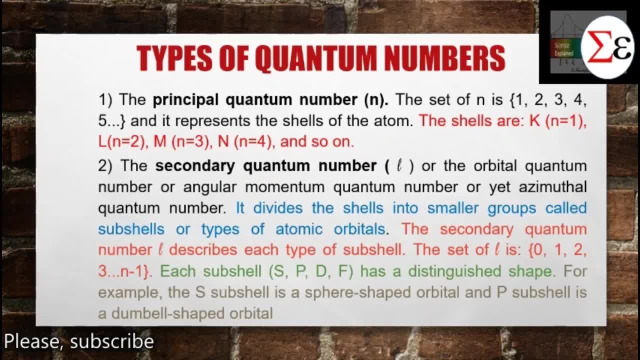 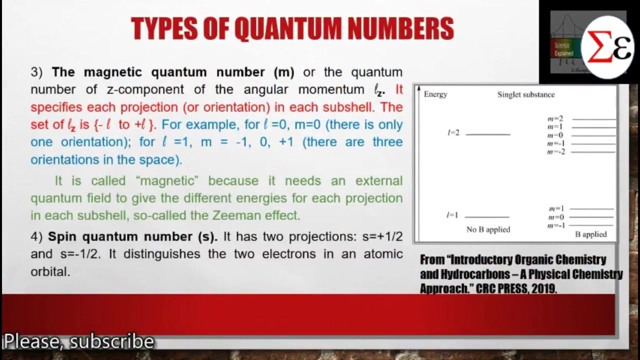 with zero, one, two, three until and minus one. each subshell named as spdf has a distinguished shape. for example, the s subshell is a sphere shaped orbital and the p and the p subshell is a dumbbell shaped orbital. the magnetic quantum number, m, or the quantum number of the z component of the angular momentum, lz, specifies each. 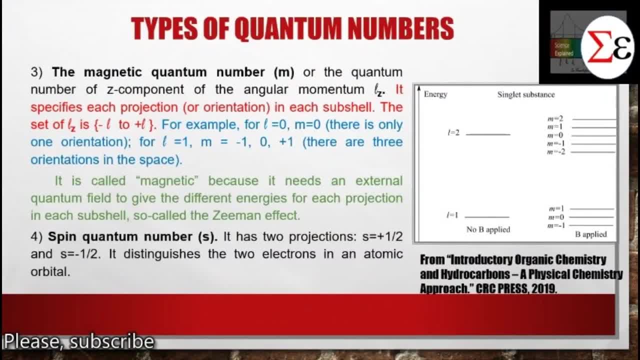 projection or orientation. in each, in each subshell, the set of lz is a set of discrete numbers, from minus l to plus l. for example, for l equals zero, m is zero, then there is only one orientation. for l equals one, m is minus one, zero and plus one, then there are three orientations in the space. 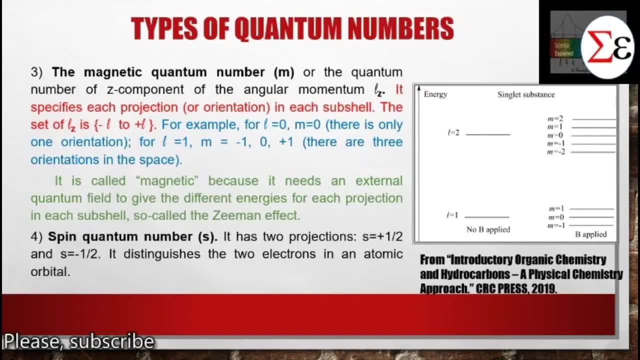 it is called magnetic because it needs an external quantum field to give the different energies for each projection in each subshell. this was obtained by the zeman experiment and it's called zeman effect. as we can see here, the uh, l one subshell and l two subshell when there is no magnetic. 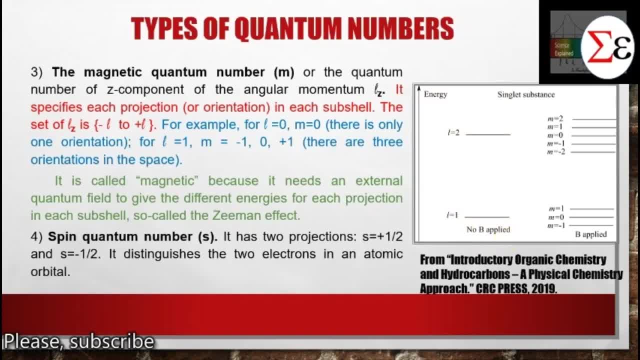 field applied to the atom and, when it's applied, a magnetic field. b. we see that the, the three orientations of the l, one subshell, is divided into three types, into three energies. three different energies for the l equals two. when it's applied the magnetic field, it is split into five. 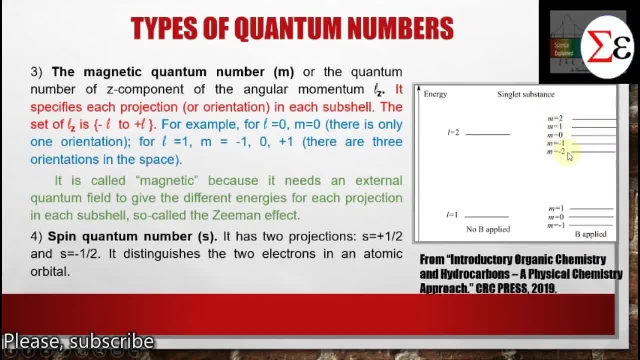 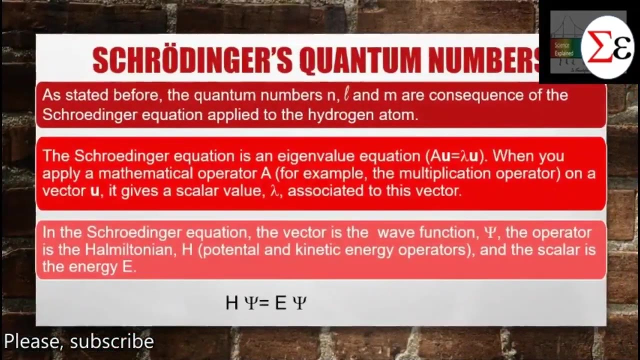 orientations of this subshell. and the fourth quantum number, the spin quantum number s, has two projections, s plus a half and s minus a half, and it distinguishes the two electrons in atomic orbital. so let's talk about the strongest quantum numbers. as stated before, the quantum numbers l. 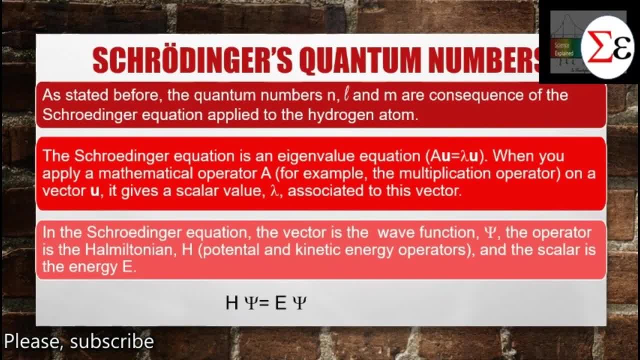 n, l, m are consequence of the shorn equation applying to the hydrogen atom. the shrine equation is an eigenvalue equation, for example, and the general equation is: a times u equals lambda times u. when you apply a mathematical, mathematical operator a, for example the multiplication operator, on a vector u, it gives a scalar value- lambda- associated to this vector. 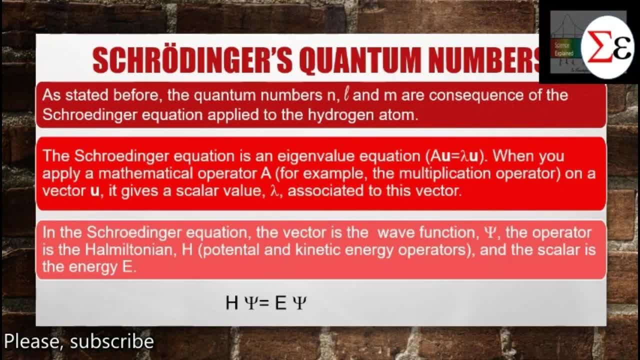 In the Schrodinger equation the vector is the wave function, psi, and the operator is the Hamiltonian H, which is the potential and kinetic energy operators, and the scalar is the energy E. The famous time-independent Schrodinger equation is this: The Hamiltonian H applied to psi gives E and the psi 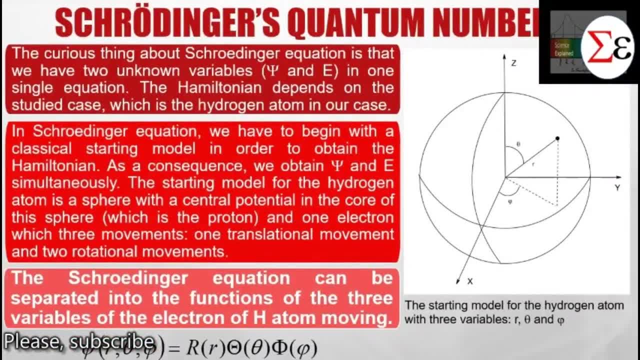 The curious thing about the Schrodinger equation is that we have two unknown variables, psi and E, in one single equation. The Hamiltonian depends on the study case, which is the hydrogen-h NOR-case. In the Schrodinger equation we have to begin with a classical starting model. 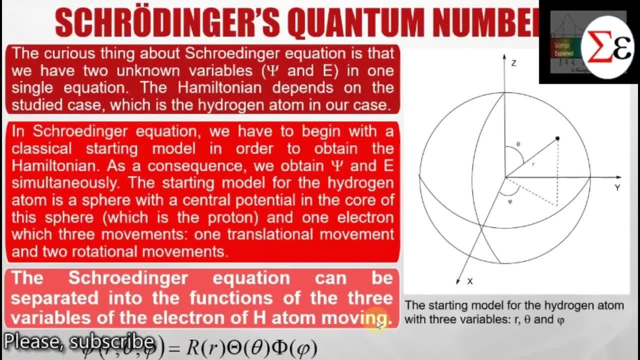 in order to obtain the Hamiltonian. As a consequence, we obtain psi and E simultaneously. The starting model for the hydrogen-h NOR-case is a sphere like this, with a central potention in the core of the sphere which is the proton, and one electron which has 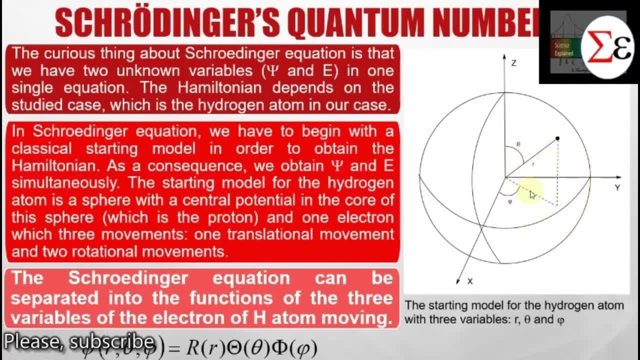 free movement, one translation-m Rolling motion, two rotational movements, where the variables are r for the translational movement angles, theta and phi. so and the strong equation can be separated into the functions of the three variables of the electron, of the hydrogen atom, which is given here. psi is a function of three. 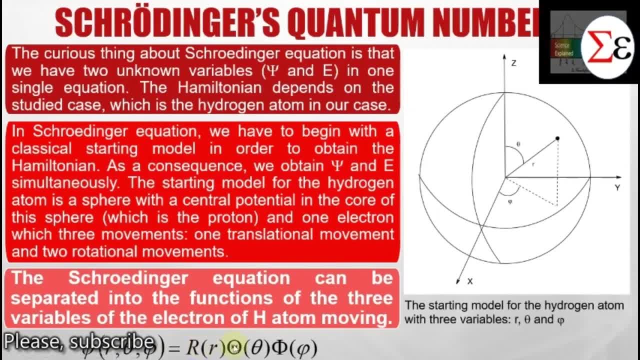 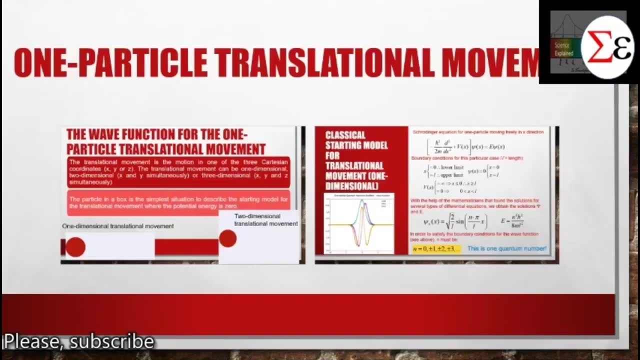 variables which can be separated into the functions of each variable: r capital letter, theta capital letter and phi in capital letter. then we go to one particle translational movement which is one of the movements of, of the electron, of the hydrogen atom. then we go to us the simplest case, that is, one particle in the 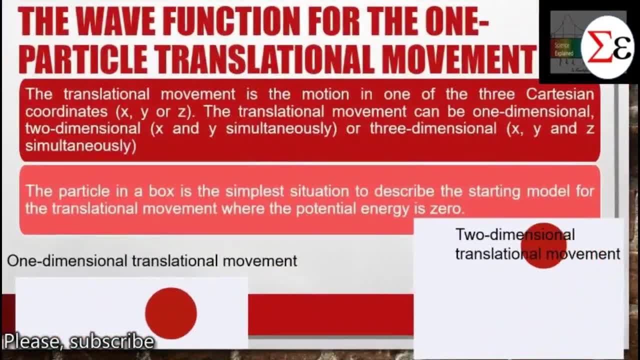 box. the translational movement is the motion in one of the three cartesian coordinates, x, y or z, and it can be one dimensional, two dimensional, where we have x and y- z simultaneously, and three dimensional, where we have x, y and z simultaneously. here we have the example of one dimensional translational movement and two dimensional 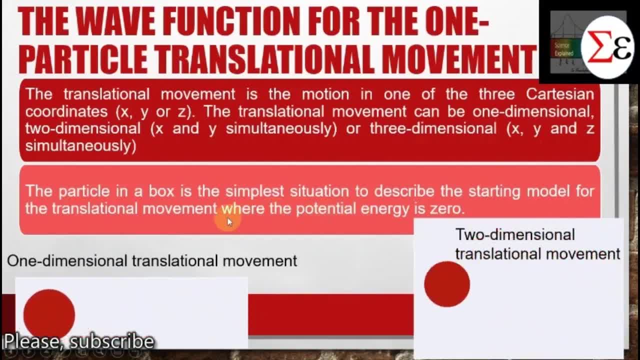 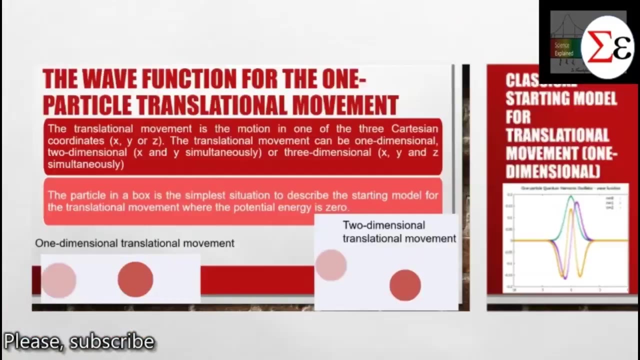 translational movement. the particle in a box is the simplest situation to describe the starting model for the translational movement, where the potential energy is zero. be attention, that is not the case for the hydrogen atom, but the results of the quantum number, the principal quantum number, n. it is partially the same. 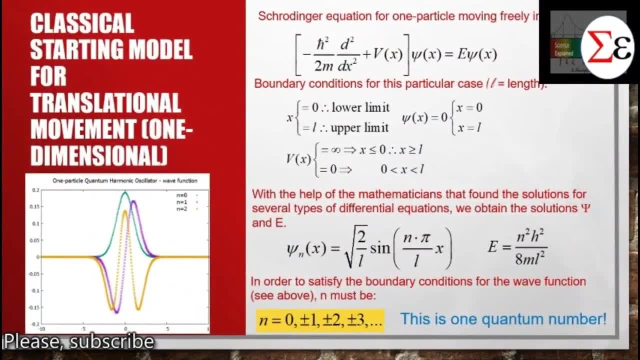 then the shrine. the equation for one particle moving freely in the x direction is given here. uh, when we say moving freely, it means that the potential energy is zero. the length of the box then, in this case, is a one-dimensional box. then we have the strand equation for one particle moving. 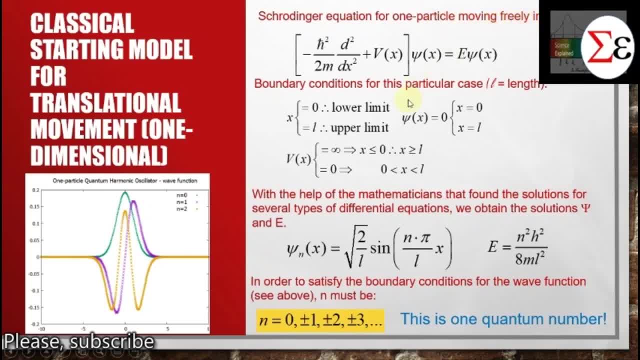 freely, which means moving with potential energy zero in the x direction, which means it's a translational movement in one dimension. then we have the shrine equation with the kinetic energy operator, the quantum kinetic energy operator and the potential energy operator, which is zero in the limit of the box. the boundary conditions for this case, where l is the length is x is zero. 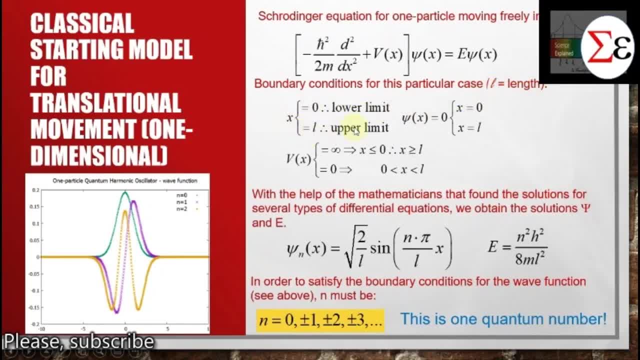 the lower limit and x is l the upper limit. the wave function psi is a function of x, which is zero when x is zero and 0 when x is l. the potential energy is infinite for x less than or equal to 0 or when x is greater than. 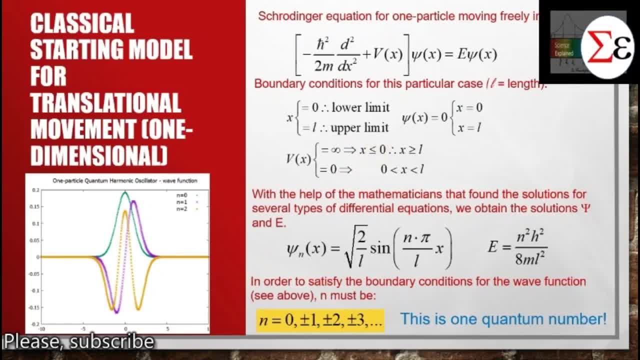 greater than or equal to L, The potential energy is zero. when X is between L and zero, Then, with the help of mathematicians that found the solutions for several types of different equations, we obtained the solutions psi and E, The wave function for the one particle. 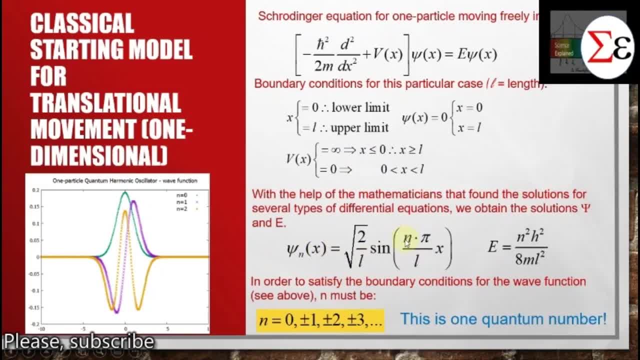 in one dimension is given here, where we have the quantum number n. In order to satisfy the boundary conditions that are given here for this wave function, n must be zero plus minus one, plus minus two plus minus three, and etc. This is one quantum number, The unique. 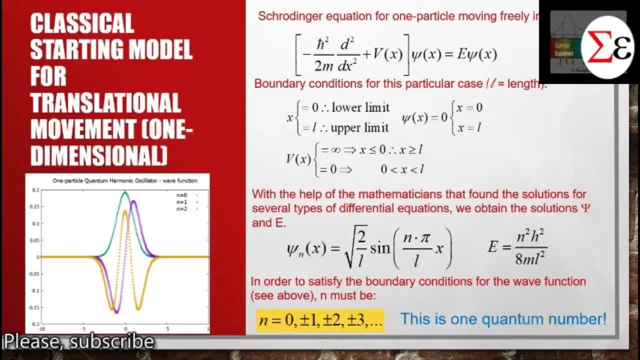 difference that we have to pay attention is that the quantum number for the hydrogen begins with one. It's only positive integers. okay, For the hydrogen atom, the principal quantum number is only positive integers, beginning with one. Here for the one-dimensional translational, 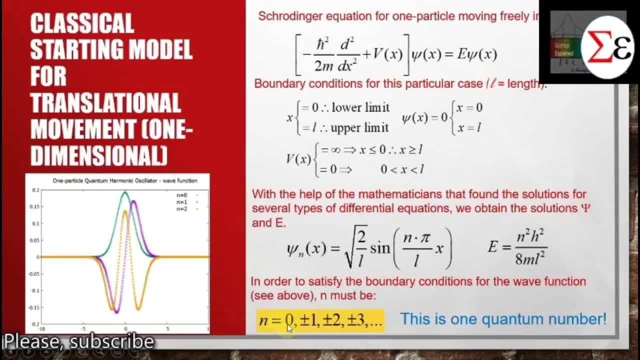 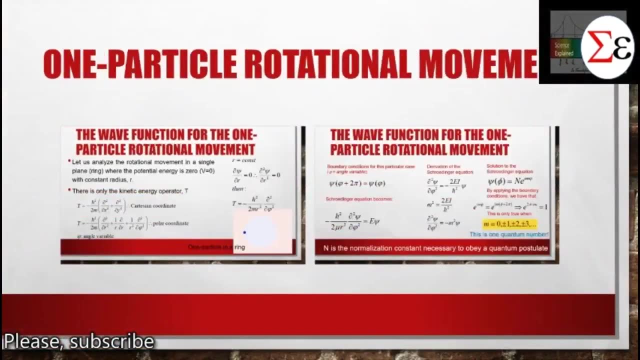 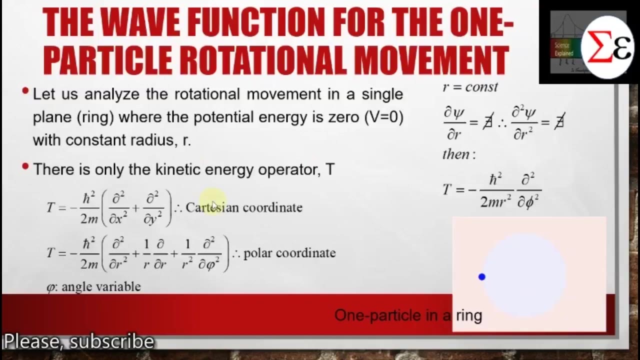 movement of one particle. we have n that can be zero and that can be negative integers. Then we go to one particle: rotational movement. Let us analyze the rotational movement in a single plane, which is the ring, as we can see here, where the potential energy is zero. 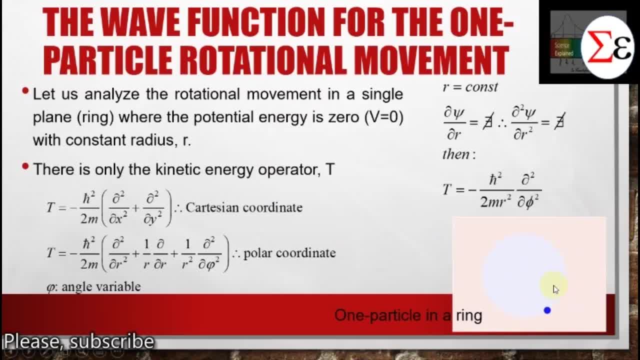 V is zero with a constant radius r. In this case we can have the same maximum energy. In this case, that is only the kinetic energy operator T. The kinetic energy operator can be described in Cartesian coordinate or polar coordinate, but it's wiser to use the polar coordinate in this case. 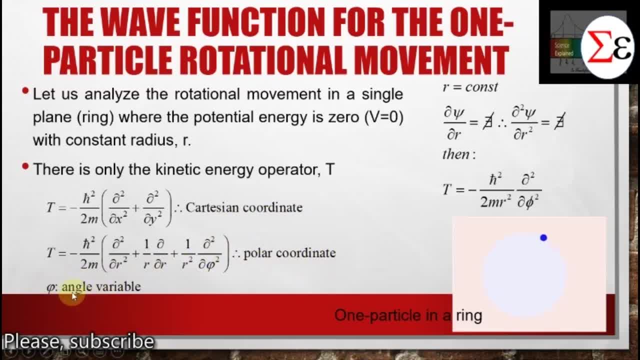 We see here the phi, which is the angle variable. Then, since r is constant, the partial derivative of the function phi over a constant r doesn't exist. The same occurs for the second derivative. Then we have a simplified kinetic energy operator. 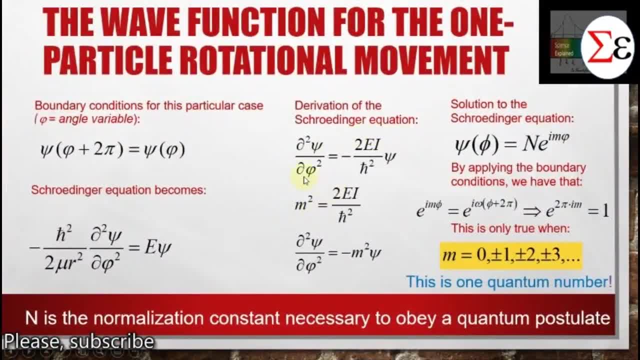 The boundary conditions for this particular case, where phi is the angle variable, is given here. When we have psi where the angle is phi, it is the same for psi where phi plus 2 pi occurs. Then we have a cycle, A complete cycle. 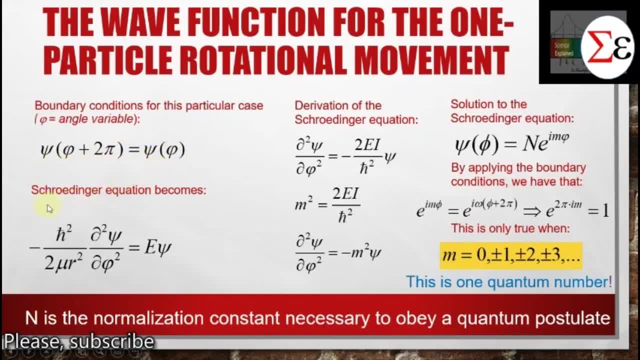 In this case the wave function is the same. Then the Schrodinger equation becomes the kinetic operator, where the unique variable is the angle phi. Then we have this derivation of the Schrodinger equation given here, and we are not interested in all the details of this derivation, but it's important to see that this part is replaced. these color numbers are replaced by this m squared. 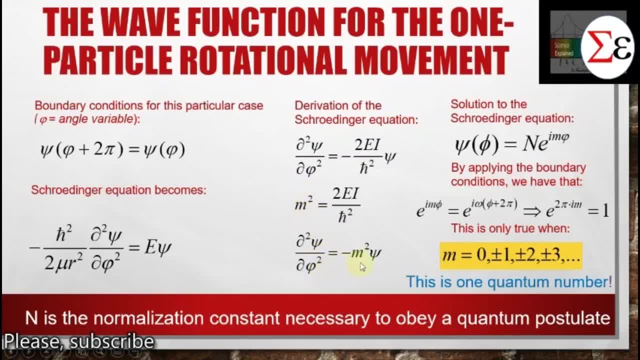 And we have this Schrodinger equation at the end. The solution for this Schrodinger equation is given here, where m is the normalization constant which is necessary to obey a quantum postulate of the probability of finding the electron within the range from 0 to infinite or minus infinite to positive infinite. 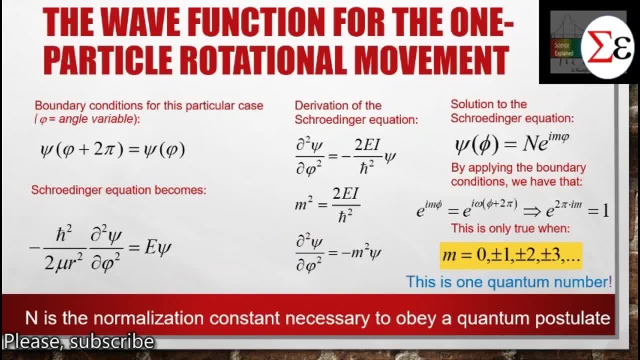 Then, by applying the boundary conditions we have, that this equation is, This part of the equation is 1.. This is only true when m is 0, plus minus 1, plus minus 2, plus minus 3, etc. 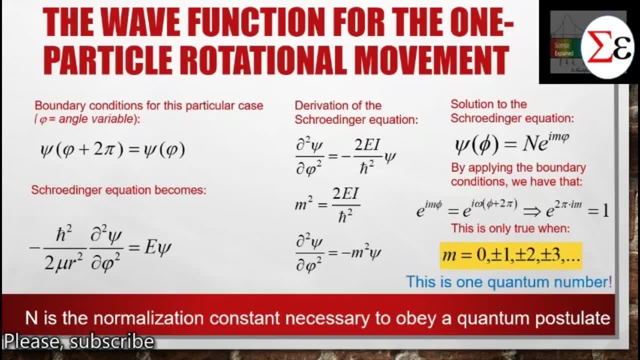 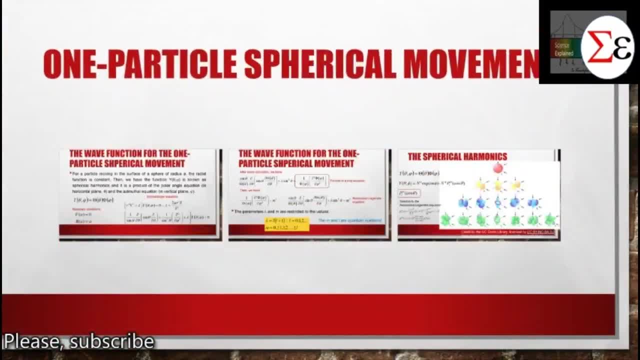 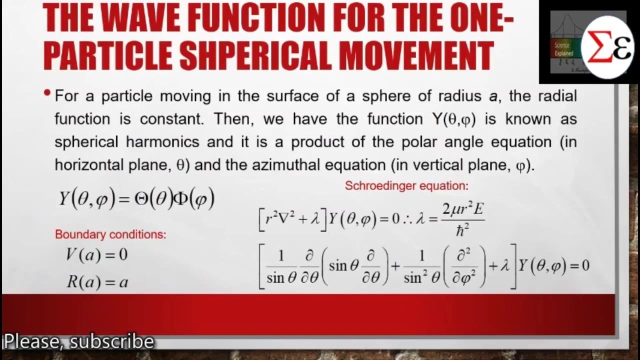 Which is the word quantum number, the magnetic quantum number Of the hydrogen atom. Then we go to one-particle spherical movement. The wave function for the one-particle spherical movement is a particle movement in a surface of a sphere of radius a, which is a constant. 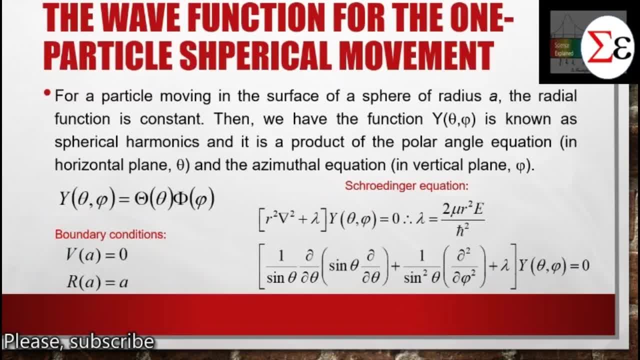 And the Potential energy is also 0, in this case, And the wave function is epsilon, or also called as spherical harmonics, And it is a product of the polar angle equation in horizontal plane, the theta, and the azimuthal equation in a vertical plane, phi, given here. 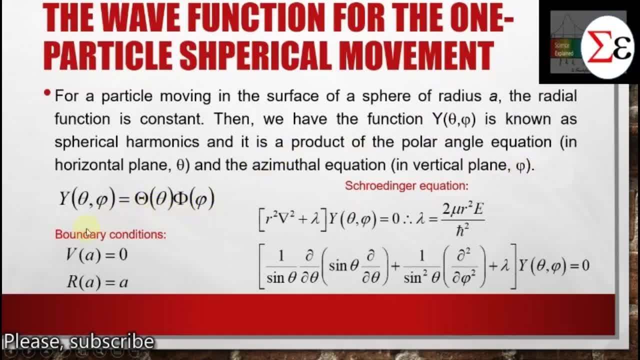 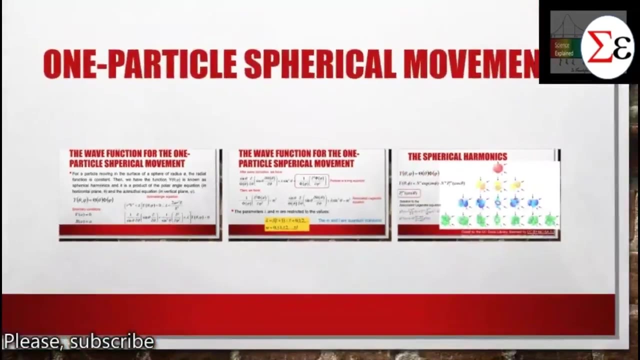 The product of the theta and phi, The boundary conditions And the corresponding Schrodinger equation where lambda is given here. Then we have this equation, the Schrodinger equation for the one-particle spherical movement. After some derivation we have this: 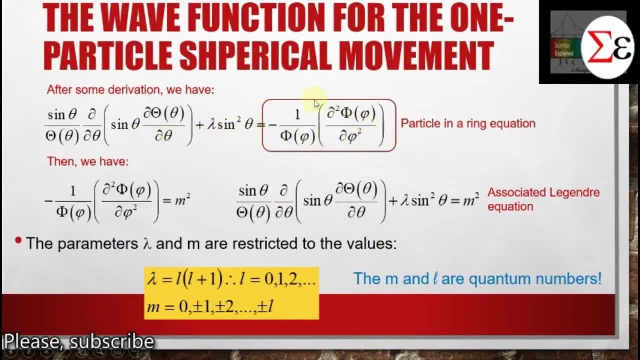 This equation, Where the second part of the equation is the particle in a ringed equation. It's similar to the particle in a ringed equation. Then, as we saw, in the particle in a ringed equation, this part this equation is the m? squared. 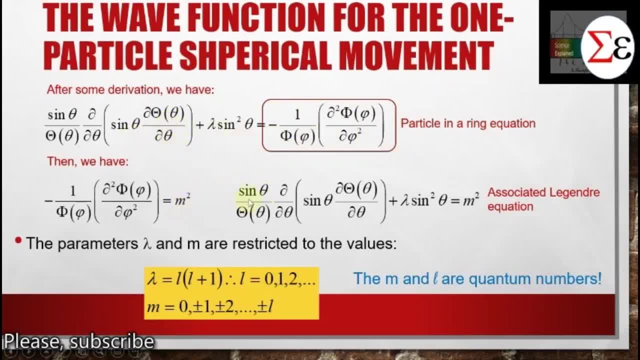 Then the first part of the equation is also the m squared, And this is associated With the Schrodinger equation, which has a well-known solution- And as a result, we have the quantum numbers lambda and m. Lambda is L times L plus 1.. 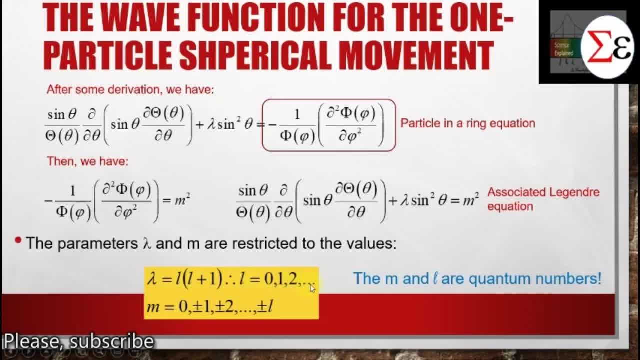 And L is 0,, 1,, 2,, 3, etc. And m is 0, plus-minus 1, plus-minus 2, until plus-minus L, And the m and L are the quantum numbers, The same quantum numbers for the hydrogen atom. 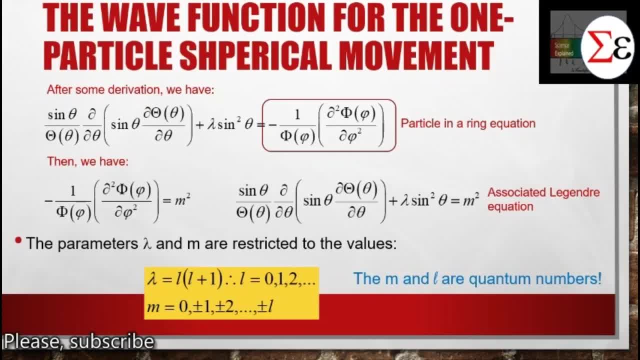 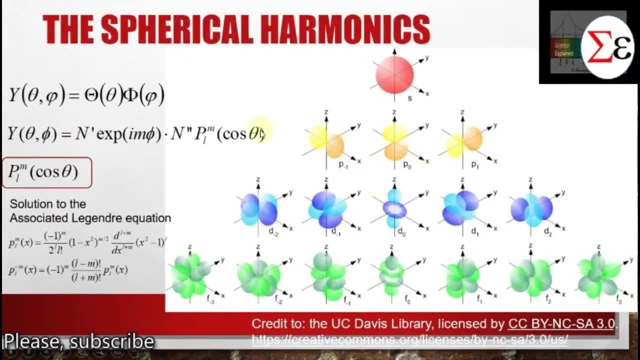 In this case it's the same. They are the same quantum numbers. The final equation is given here. Where it's missing the values for the normalization constant for the theta And the normalization constant for the phi. But we see, here is the solution for the associated legend. 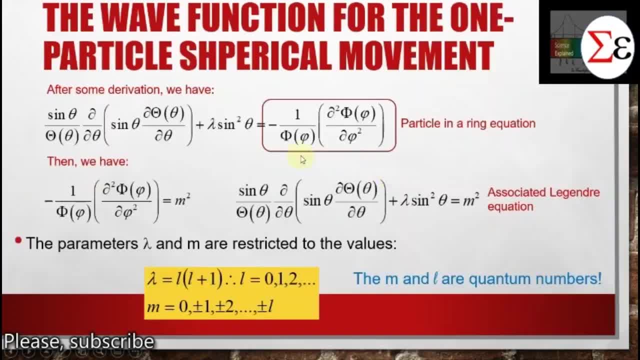 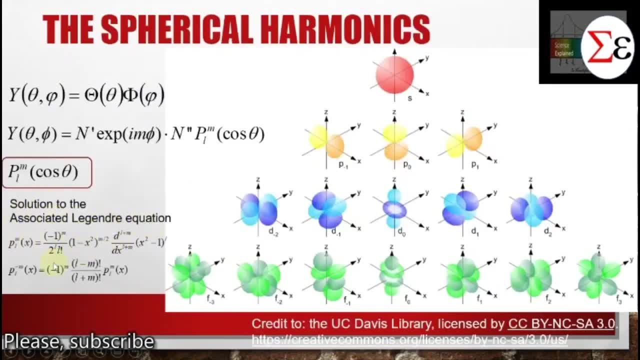 And the equation of the first part of this equation And the solution of the associated legend equation is given here. Where m is a positive, we have this solution And when m is a negative, we have this solution As a consequence of the product of the theta and phi equations. 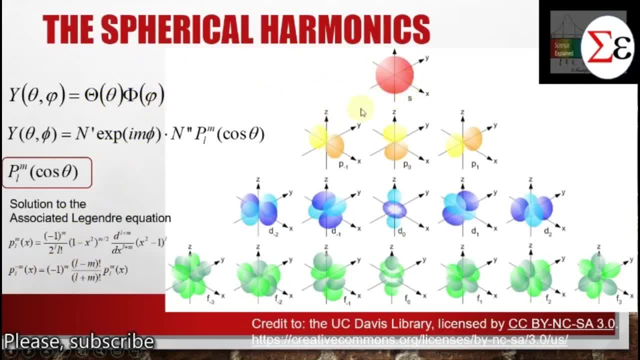 we have the spherical harmonics, Or, as we know, the atomic orbitals. Then, when L is 0,, we have the s orbital. When L is 1, we have the p orbital with 3 orientations. When L is 2,, we have the d orbital with 5 orientations. 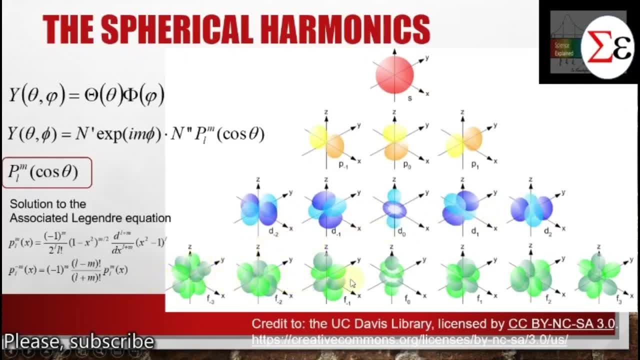 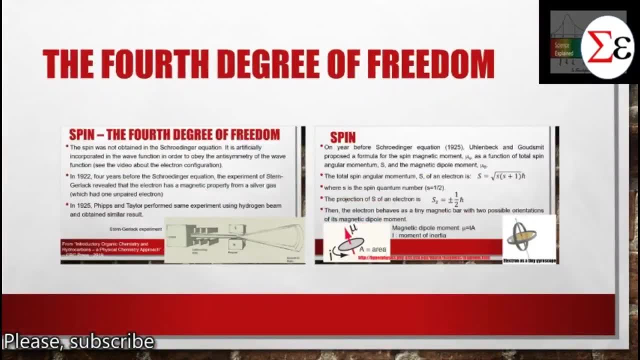 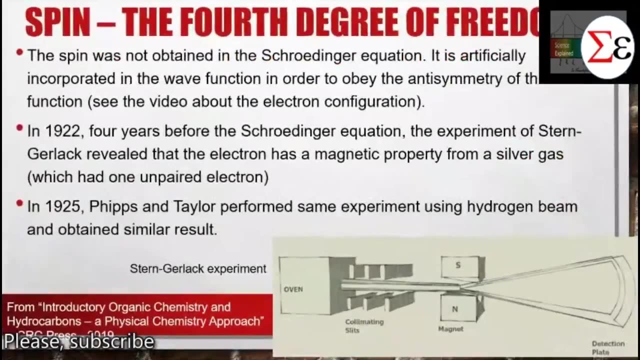 When L is 3, we have the s orbital with 5 orientations And we have the f orbital with 7 orientations. Then we go to the fourth degree of freedom, The spin. The spin was not obtained in the Schrodinger equation. 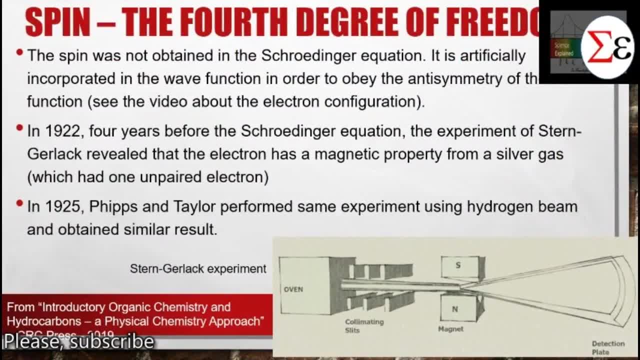 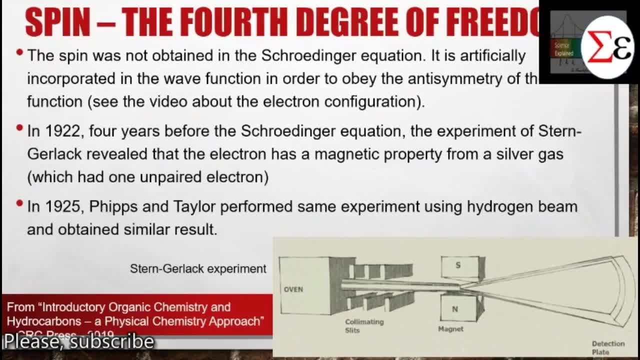 See the video about the electron configuration in the end of this video. See the video about the electron configuration in the end of this video. In 1922, four years before the Schrodinger equation, the experiment of Stern-Gerlach revealed that the electron has a magnetic property from the silver gas, which has a 1. 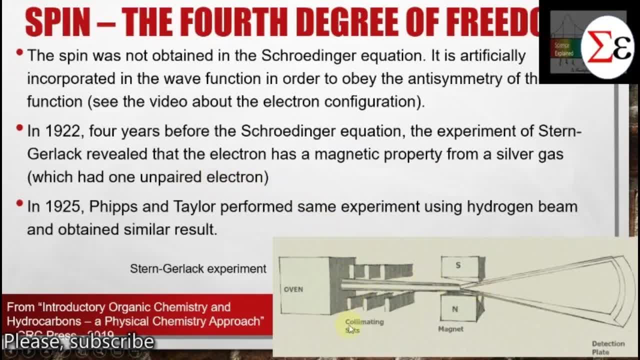 Ampere electron passing through collimator slits and the magnet, the two poles of the magnet, The two poles of the magnet, The two poles of the magnet deviated. It has two deviations, which is detected in this plate. Then is the first. 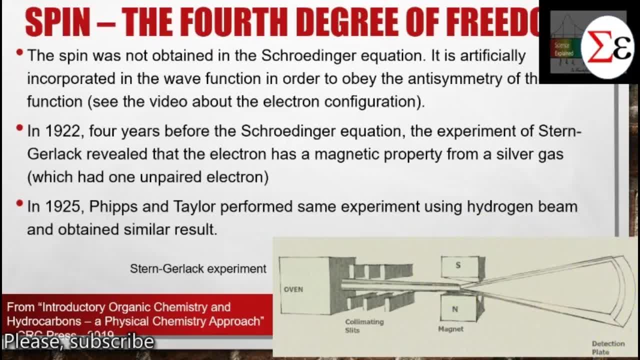 evidence of the anomalous Zeeman effect. In 1925, Phipps and Taylor performed the same experiment using a hydrogen beam which also has one unpaired electron, and obtained a similar result One year before Schrodinger's equation, which 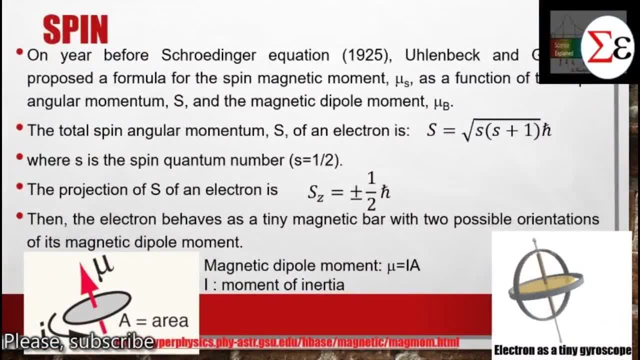 was then 1925, Uhlenbeck and Goldsmith proposed a formula for the spin magnet: magnet As a function of the total spin angular momentum S and the magnetic dipole moment mu B. The total spin angular momentum S of an electron is given by this equation, where S is the 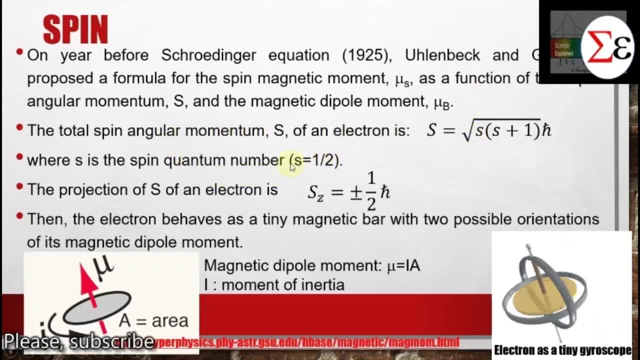 spin quantum number which is one half. The projection of the S of an electron is given by this equation. It has two projections, which are the two deviations of the silver gas beam, and then this represents the two projections of the spin. And here we see the pictorial representation of the magnetic dipole moment, where the 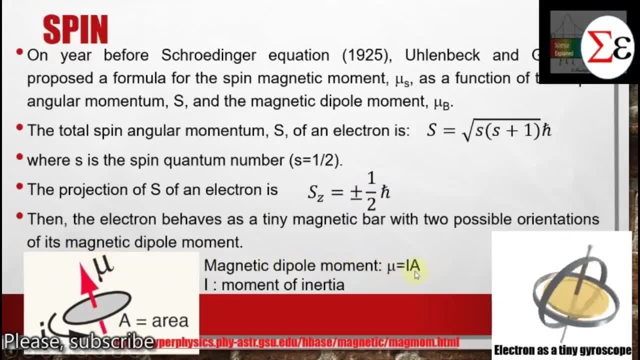 magnetic dipole, moment is mu as a function of the moment of inertia and the area. A similar result is applied to the final situation. This is to provide acribing for a squared moment of the magnetic dipole, and then the released moment is mol. times, thinkand the. 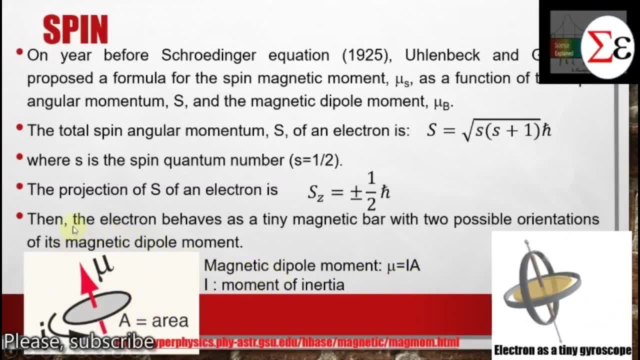 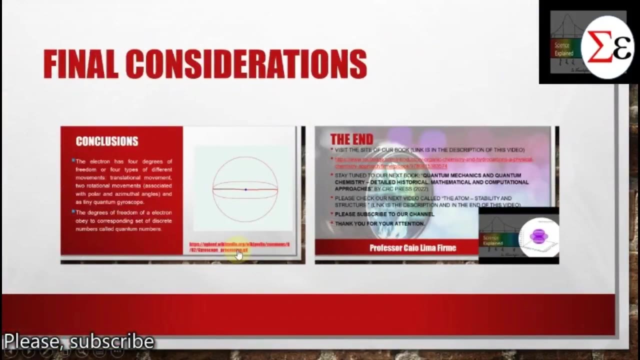 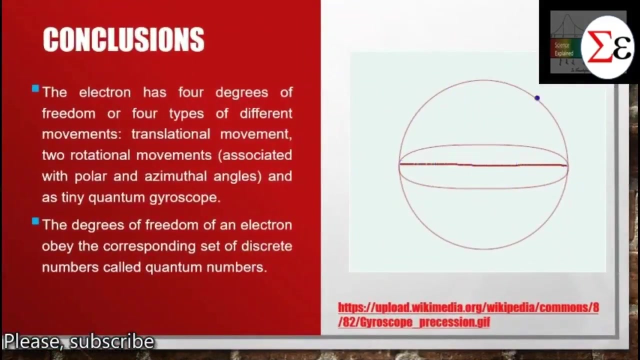 the magnetic dipole moment of this pin. Then the electron behaves as a tiny magnetic bar or a tiny gyroscope with two possible orientations of its magnetic dipole moment. Finally, we come to the final considerations. Then we conclude that the electron has four degrees of freedom, of four types of different. 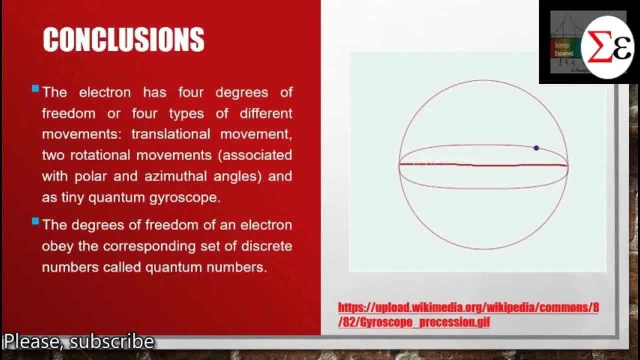 movements: Translational movement to rotational movements associated with the polar and azimuthal angles and the movement of the tiny quantum gyroscope. The degrees of freedom of an electron obey. the corresponding set of degrees of freedom of an electron Obey. the corresponding set of discrete numbers called quantum numbers.